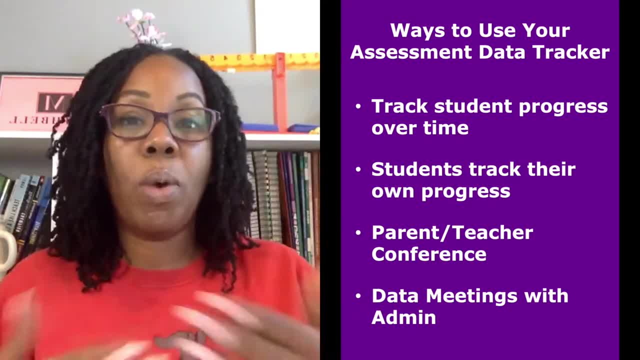 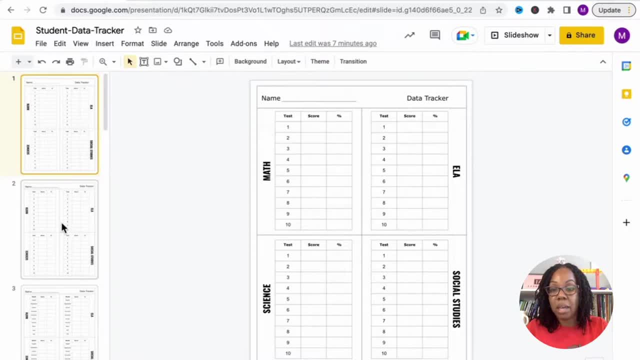 it with your resource team or your administration, to show what's going on with your students at that specific point in the school year. Let's look at some examples of what you can actually create here in Google Slides. So I have this main one where you can track. 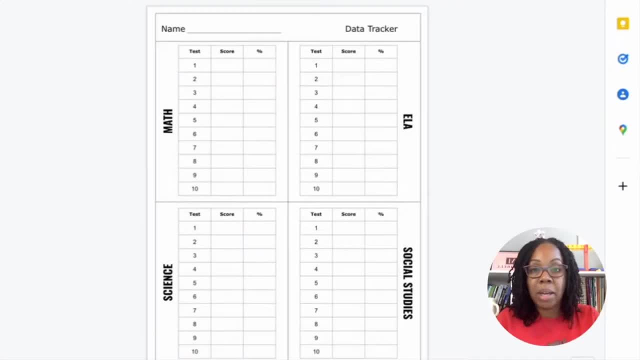 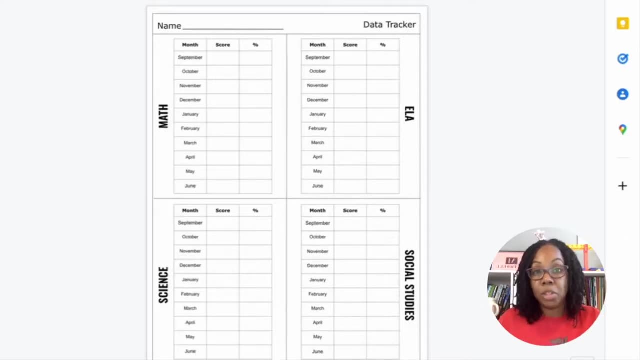 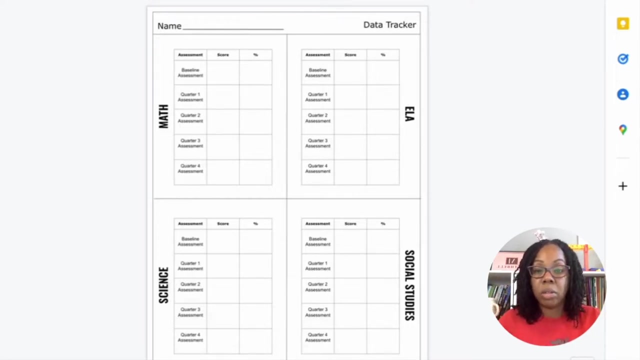 10 assessments during the year. This is by number, or if you teach August to May and you want to track it that way, or if you teach September to June and you want to track it that way, Maybe your students only take four assessments throughout the year, quarterly or even. 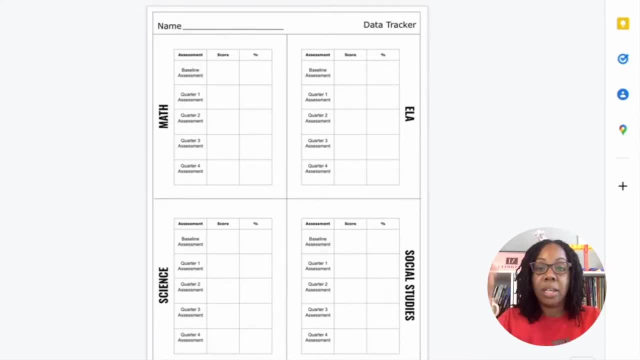 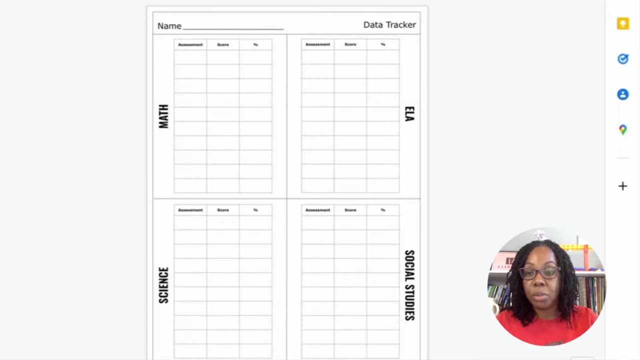 if they do like three tests, if it's like a diagnostic test and you want to track it there as well, you can do that. You can leave it blank. if you want to write on it, or if you want to do just one subject on a page and have it all written out, you can adjust it based on what you want. So 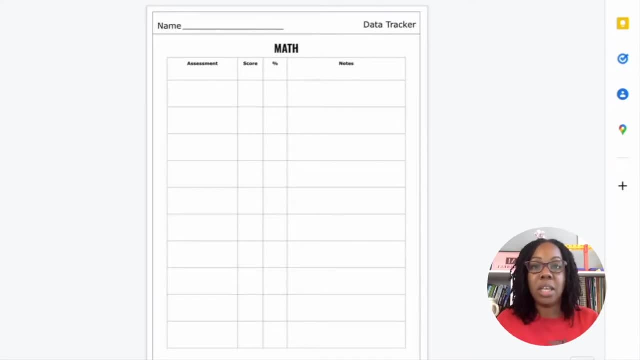 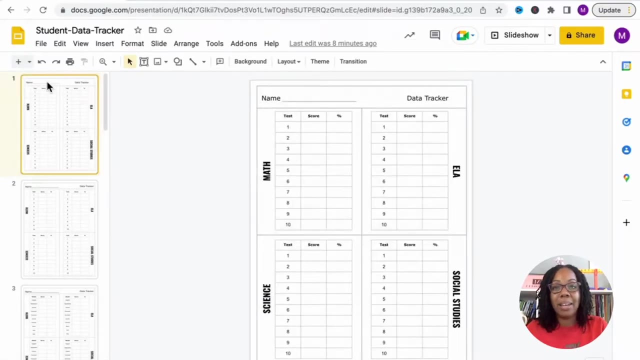 this is showing you the basics of how to set it all up, and then you can adjust it based on what goes on in your classroom and what goes on at your school. So let's get started by adding in a blank slide. We're going to go to the plus sign up here. 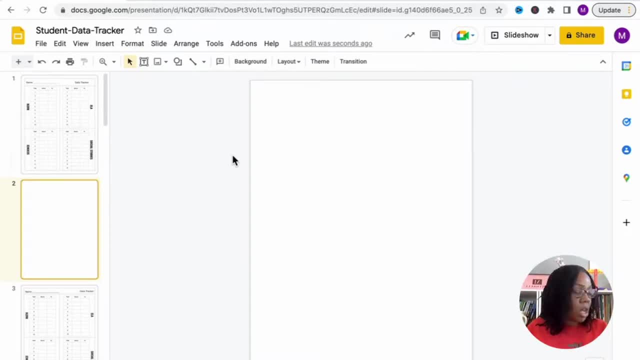 I have my notes next to me so I can keep track of what we're doing in what order. So we're going to start out by adding in a rectangle. so you're going to go up to the shapes tab and click on a rectangle. I'm going to be zooming in and out a lot just to make sure certain things need. 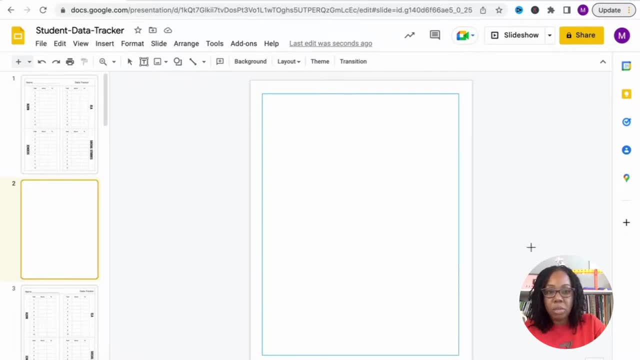 to be precise, certain things don't. so get your rectangle how you want it, and I'm going to go ahead and change the color to black just to make that line pop out, and then you can move it up and down to make sure it's centered. 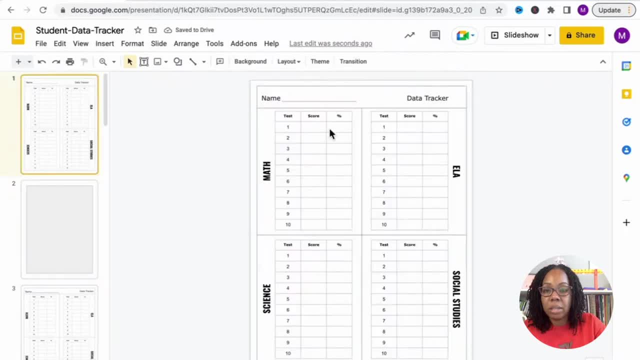 Next we're going to add in lines. so, like the lines here, we're going to add in intersecting lines here and then a line to go at the top for our heading. So we're going to go back up to the tab here and go to line. 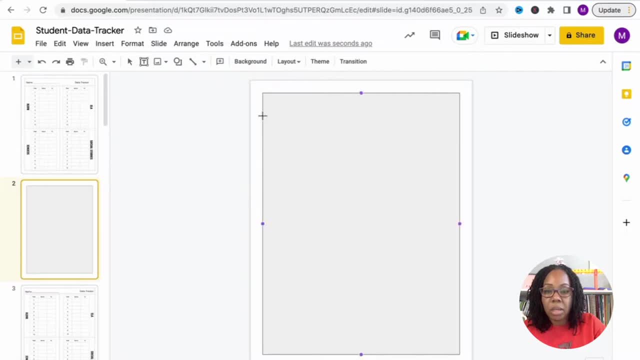 and click on line, then I'm going to do one here for the heading, and then let's change that, make sure it's black, and then I'm going to: let's zoom in now so we can make sure it's all the way on the edge. 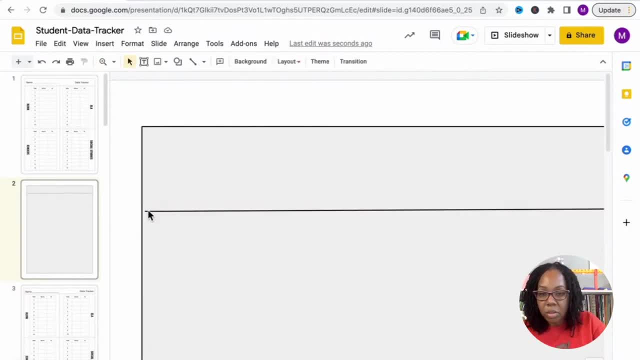 So you see, here it's a little bit short. so I'm going to zoom in, even where I'm going to extend that line, and then go to the other side and shorten it here, decrease it on this side. all right, that works, let's zoom back out. 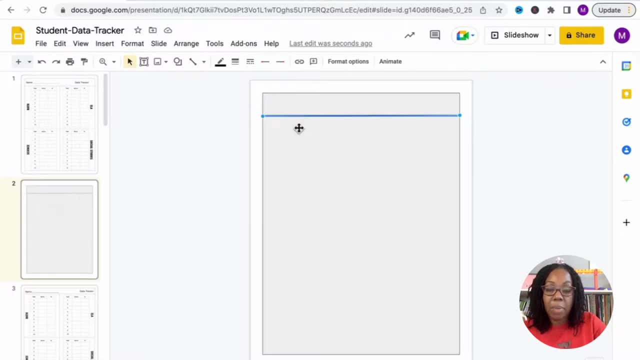 so I'm going to take that line and I'm going to hit command d on my keyboard. you can hit control d if you have a pc. I'm just going to bring it down here. you want to make sure the top and bottom sections are about the same. 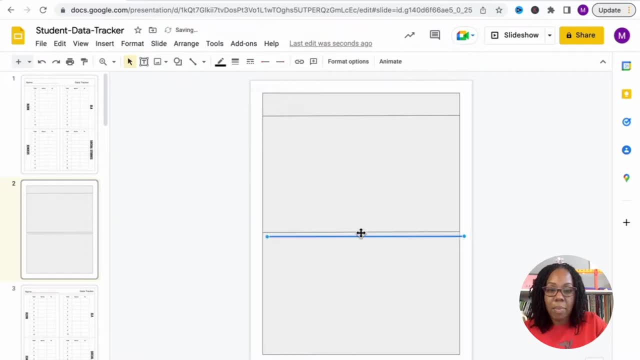 all right. so now click back on that line and hit command d again, and we're just going to change the direction of the line so that we have our vertical line going up and down the page. so I'm going to make sure it's straight by clicking on that purple dot up. 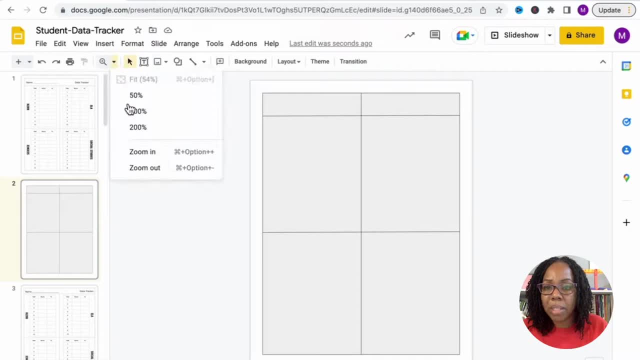 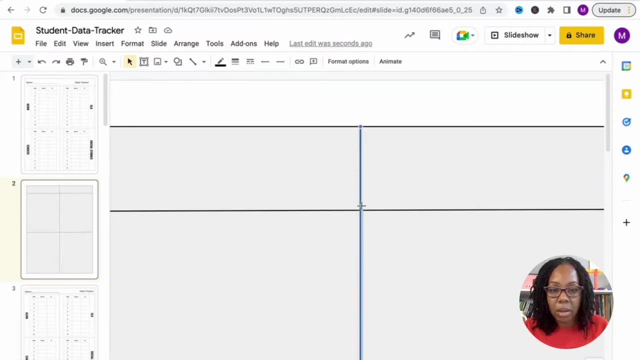 there, but then I'm going to bring it down because I don't want that partition in the heading section. so I'm going to zoom in, bring this down, make sure it's lined up. all right, that's good for me. let's zoom back out. okay? so there's our setup. so next we're going to be adding in our tables. so just to double. 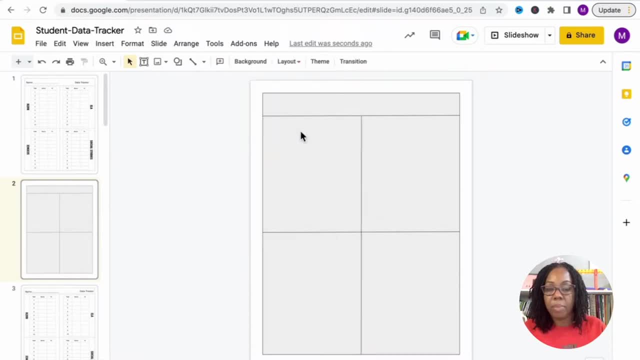 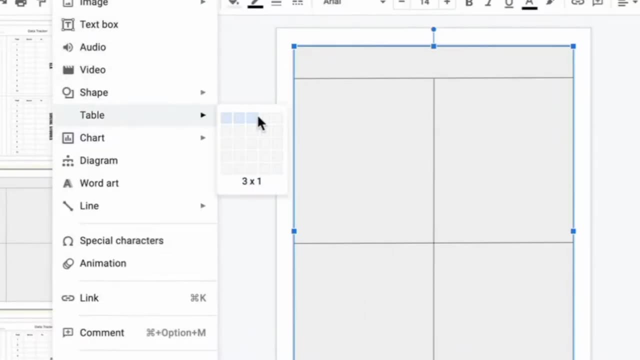 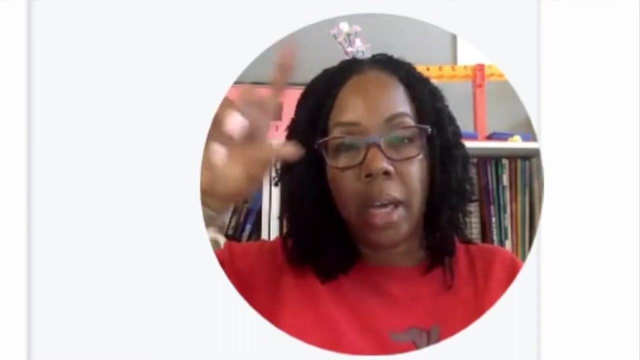 check that those lines are all black. okay, great. so now we're going to go up to the ribbon and click on insert, go to table, and I want 10 spaces for each side test, and then I'm going to add another one for like the labels. so we want 11. 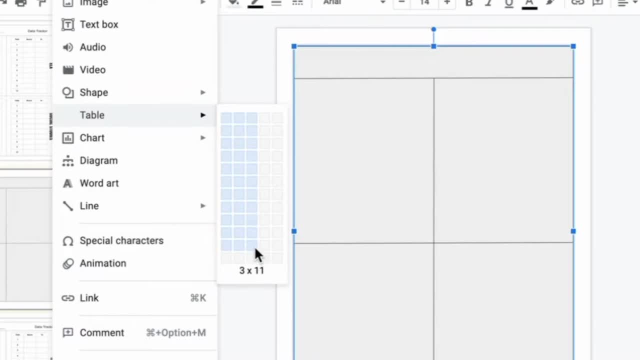 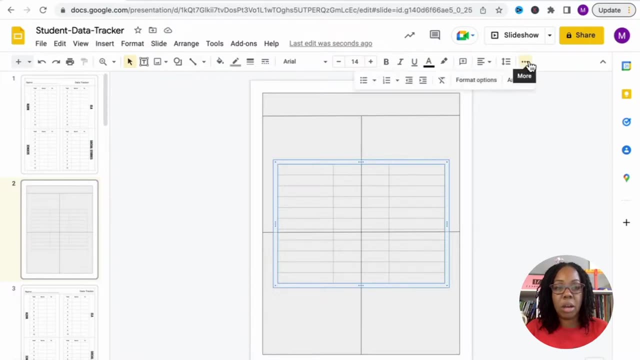 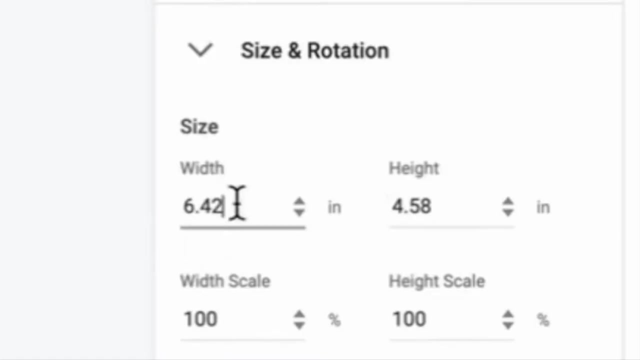 rows and three columns. before I move this around, I'm going to click up here in the more section, or these three dots are, and we're going to go to format options so we can reshape our table. so where it says with, I want it to be about: 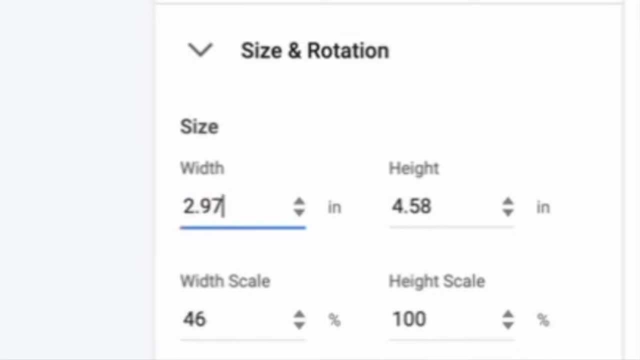 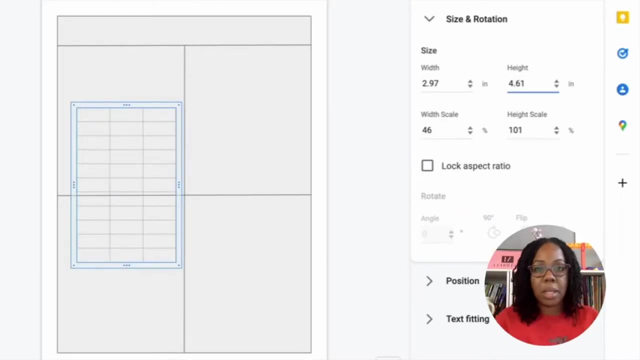 two point nine, seven inches, and then the height to be four point six, one, that's not. you don't have to make it exactly that or around that. this will work on. resize it to fit how many sections you have or how many cells you have. you might have more or less than I do, all right, so let's highlight this. 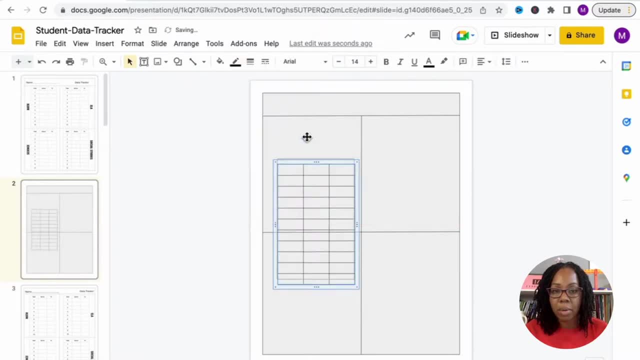 change the lines to black and now we're going to move it up. I do want it closer to the right side or towards that middle vertical line, because on the edges here we're going to put our subject labels. all right, that looks good. let me resize the font and see if that makes our table look a little bit. 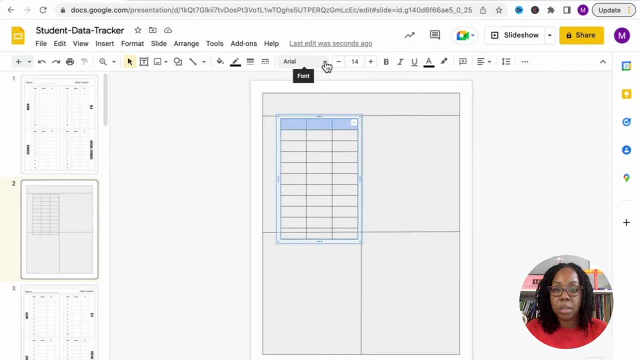 different. so at the top I know I want it to be for Dana and we're going to make it ten and we're going to Center it. so those labels and put them in the middle. so I'm going to type in test- hope you want it to be bold, test. I can zoom in so you. 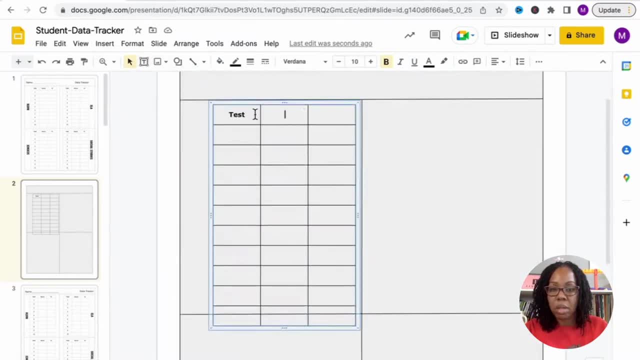 can see better test score and then the percent sign. all right, everything is all right. so we're going to put our numbers and we're going to Center them, all right. so one, two, three, four, five, six and so on. okay, so right now my table is not fitting, and it's more so likely because 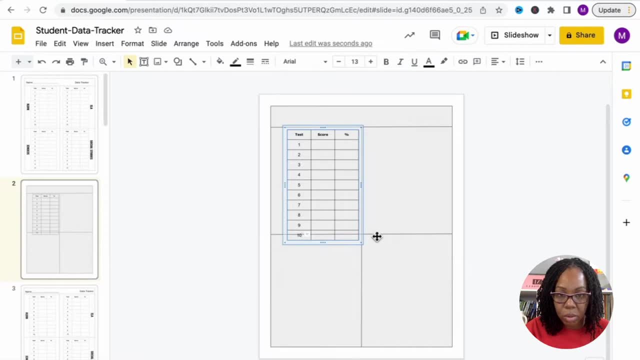 my line here is too high and the one up here is too low, so now I'm going to move it, see if it fits. it fits a little bit better. this line is a little bit short now, so I'm going to just adjust that really quickly. now we have our table and 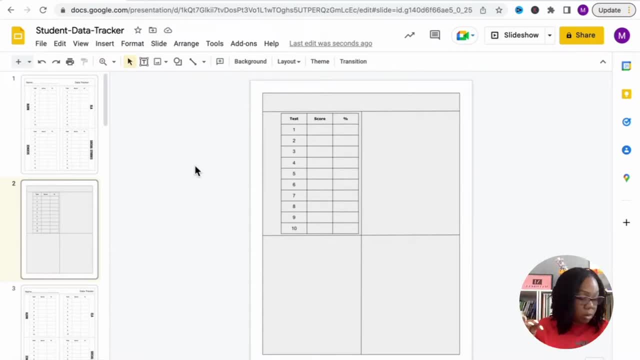 now we're going to add in, or we added in our labels. now we're going to duplicate our table. so I'm going to select the table and, just like I duplicated the lines, I want to hit command D or ctrl D and move that over so it's lined up, and make sure it's where I want it to be. I think they're a. 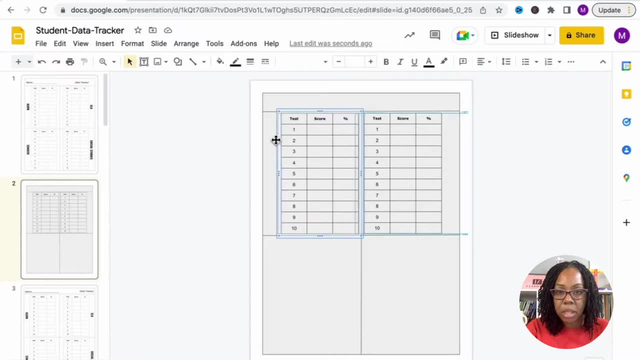 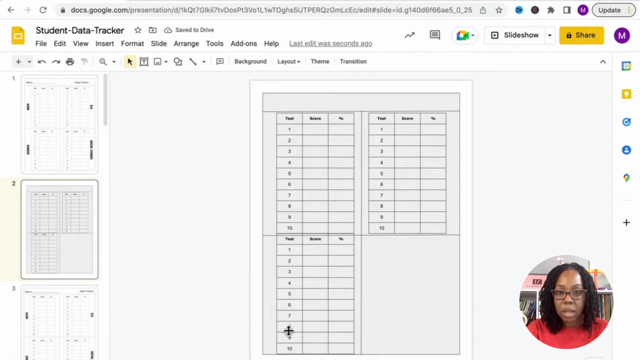 little bit too far over, so let's move that over them just slightly to the left. yeah, that looks good. all right, so we have our two top subject tables. select our table again and we're going to hit command D to duplicate: bring it down. so it's lined up. let's look here. okay, our rectangle is: 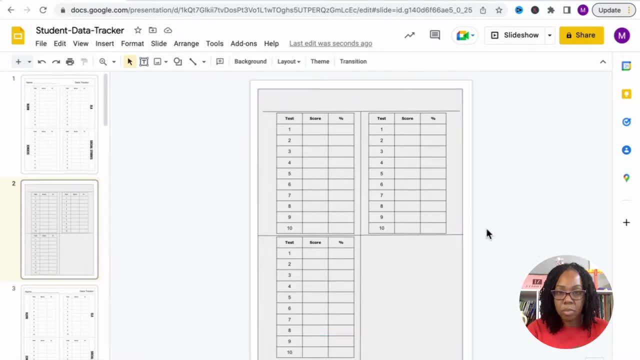 a little bit too long, so we're going to move it over here and we're going to. so the bottom of the rectangle looks like this, so I'm going to make sure that we're okay with that. it's not too small, so we're just going to adjust that all. 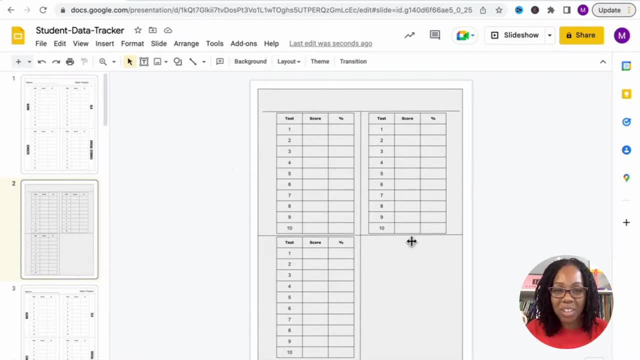 right, that's a little bit better, and if you want to make any more adjustments, go right ahead. you can definitely do that. okay, so I'm gonna take my table on the bottom and then hit command D again to duplicate, move it over and we have our four tables. they're in a good spot. so now we're going to add in our labels for: 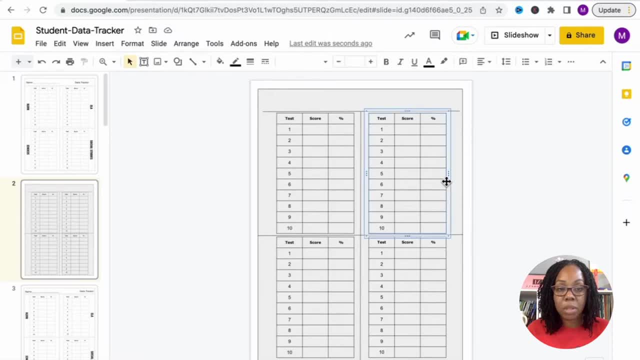 each subject. so whatever subjects you want to focus on, you can label them. you're going to label them on around the edges, and if you teach one subject, you can do multiple class periods if you want. okay, so what we're going to do is go to the 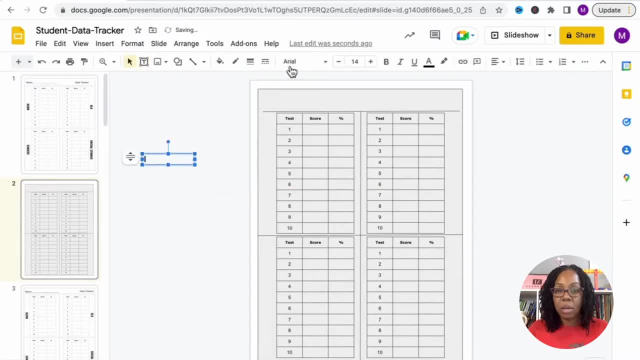 text box and make it here, change your font and your size, alright, so I'm going to do mine in all caps- math, that's the opposite of all caps. there we go and we're going to Center it. alright, let's bring this down. so it's going to go here. 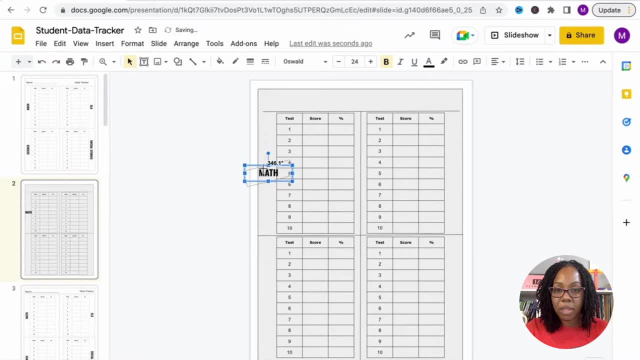 around the five or the fifth assessment. we're going to rotate that, alright. so there's math. so while it's selected, we're just going to hit command D and move that one down for our next subject. hit command D again, bring it over to the other side and then 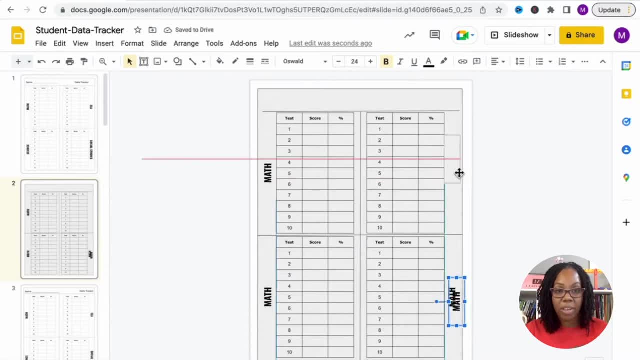 hit command D one last time for now to get in our last subject over here. so switch it to the subjects that you need. so this one's going to be ELA, this one's going to be science and this one's going to be social studies, if anything goes. 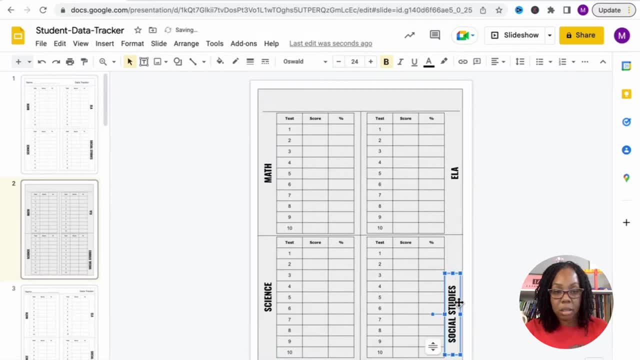 longer. you're just going to extend your text box. you're just going to extend your text box and then adjust the positioning of the text box. last we can rotate. my buttons are not working for me today. I think I know why I was using when I was working on this earlier. I wasn't using. 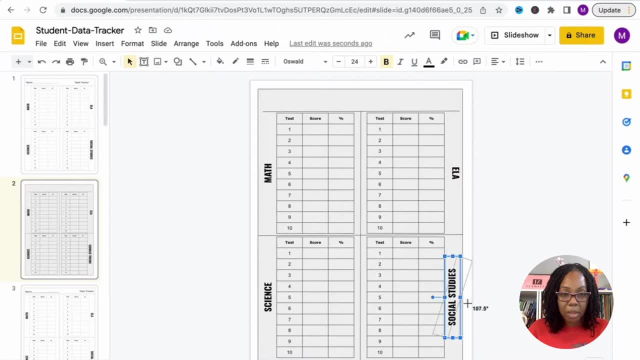 my mouse. I was using the pad on my- my mouse. I was using the pad on my- my mouse, I was using the pad on my laptop, so it's easier to maneuver with, or laptop, so it's easier to maneuver with, or laptop, so it's easier to maneuver with, or. so I thought, okay, so we have all our. 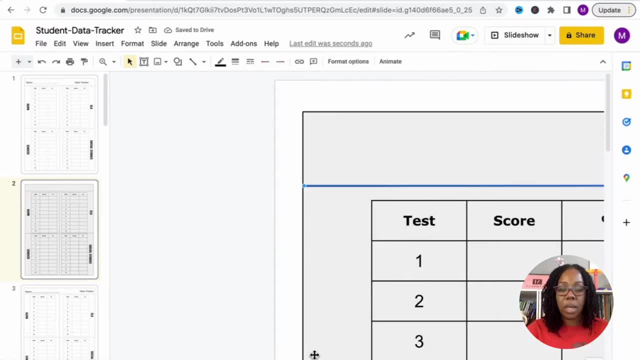 so I thought: okay, so we have all our. so I thought: okay, so we have all our subjects. those are in place now. so to subjects. those are in place now. so to subjects: those are in place now. so to get our label for our name and send. get our label for our name and send. 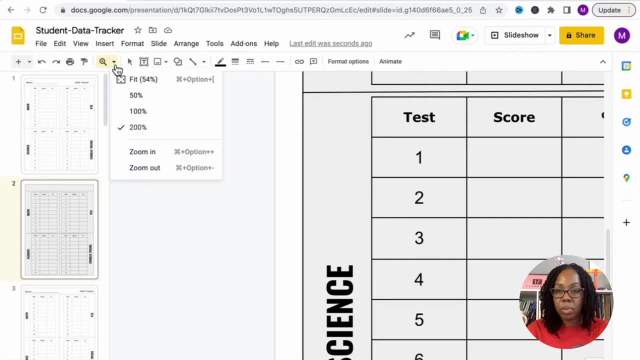 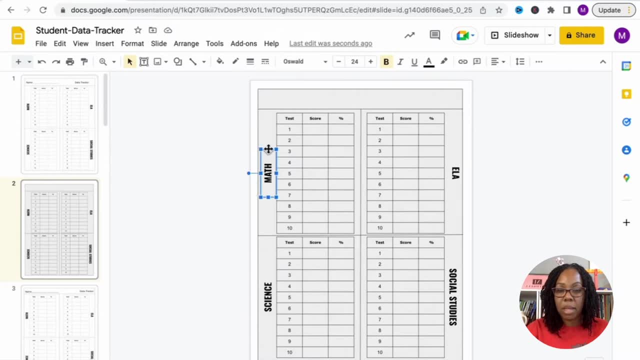 get our label for our name and send back out. going to grab the text box for math back out. going to grab the text box for math back out. going to grab the text box for math- duplicated, duplicated, duplicated, duplicated, duplicated and then move it up here you can start with the new text. 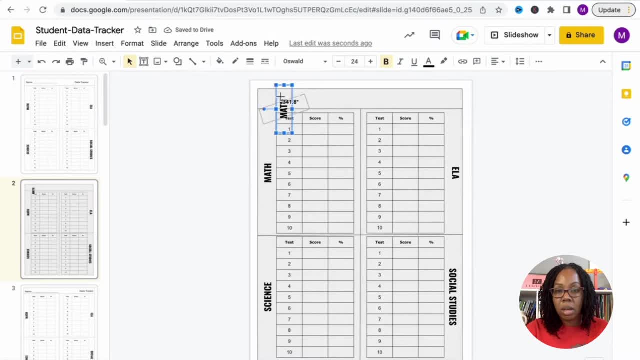 and then move it up. here you can start with the new text and then move it up. here you can start with the new text box, if you want it really box, if you want it really box, if you want. it really doesn't matter, and we're just going to change. 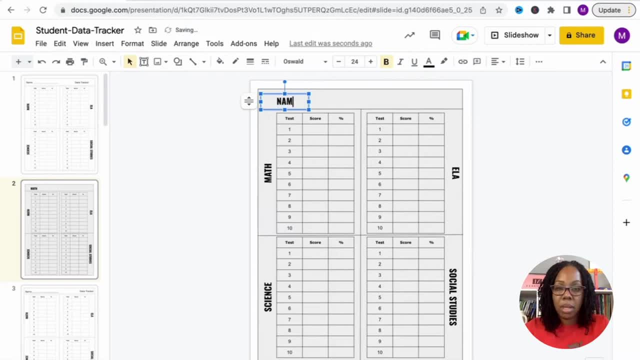 doesn't matter, and we're just going to change, doesn't matter, and we're just going to change the font and the text. so it's the font and the text. so it's the font and the text. so it's going to be named, going to be named. 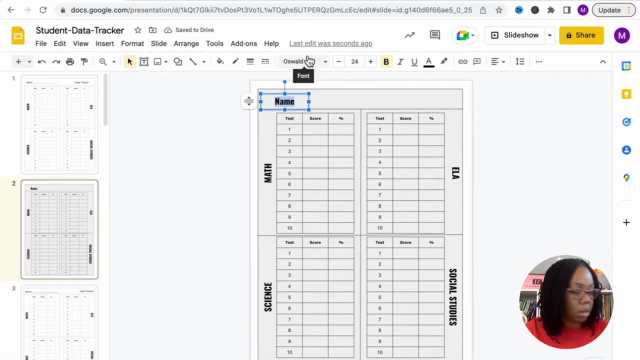 going to be named and we're going to move it over then. and we're going to move it over then. and we're going to move it over then. we're going to add a line for them to. we're going to add a line for them to. 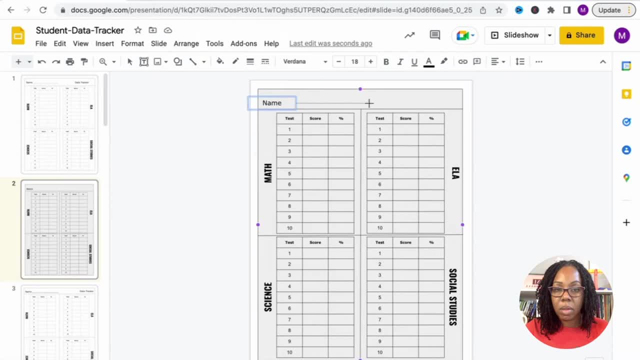 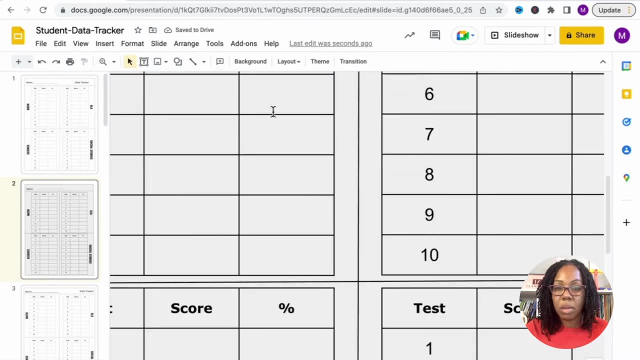 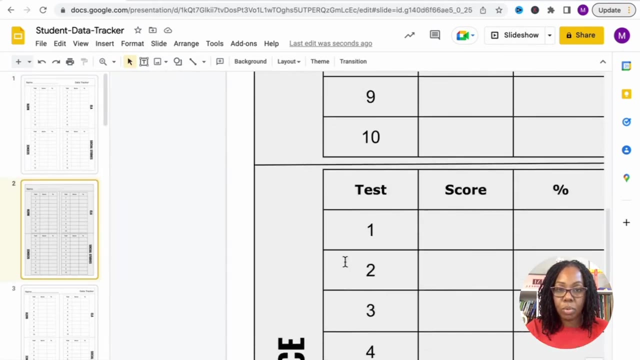 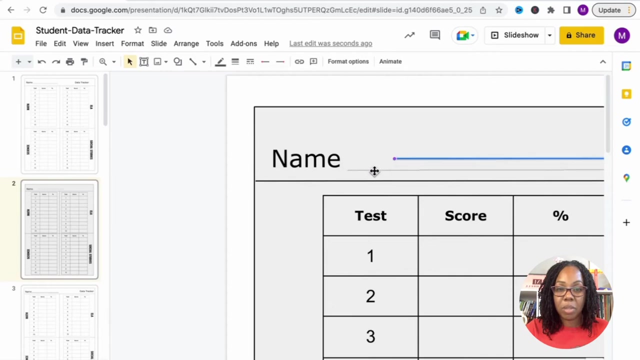 we're going to add a line for them to write their name. and let's zoom in: write their name. and let's zoom in: write their name and let's zoom in. singing a song that plays in my Zumba. singing a song that plays in my Zumba. 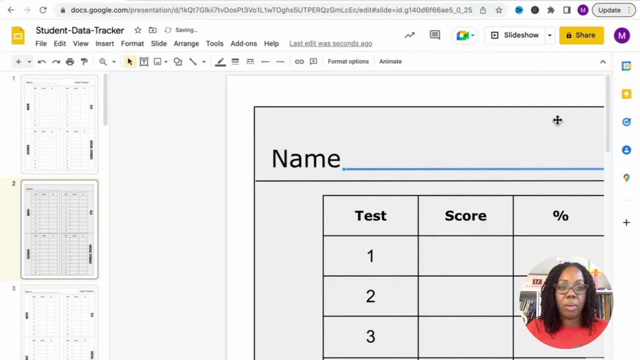 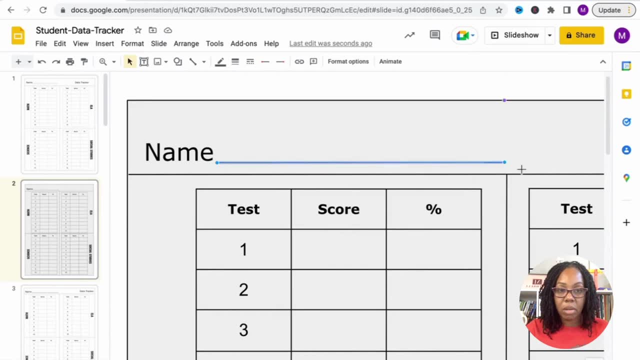 singing a song that plays in my Zumba class. all the time songs are in your class. all the time songs are in your class. all the time songs are in your head now. all right, that's looking good head now. all right, that's looking good head now. all right, that's looking good. looking good, looking good, all right. a. 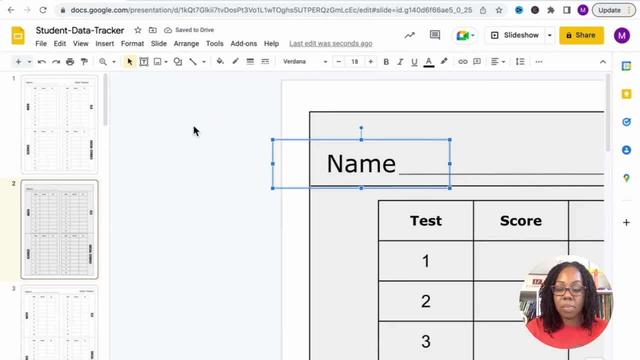 looking good, looking good, all right. a looking good, looking good, all right, a little bit more, okay. so let's take the little bit more. okay, so, let's take the little bit more okay. so let's take the name text box duplicate that we're gonna. name text box duplicate that we're gonna. 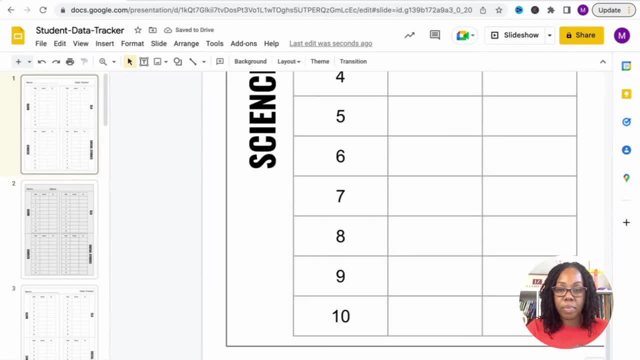 name: text box: duplicate that. we're gonna move that over, move that over, move that over, over, over over you. my computer is going so cuz I'm you. my computer is going so cuz I'm you. my computer is going so cuz I'm recording it. this is what happens when I 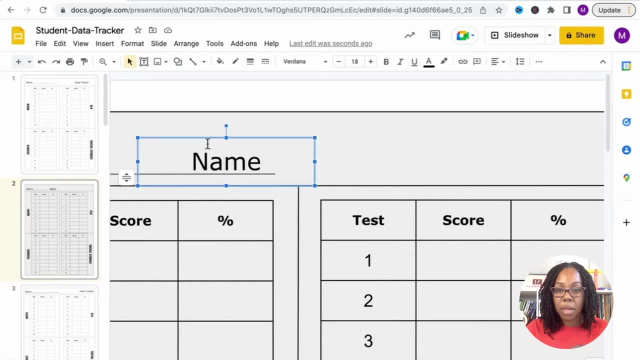 recording it. this is what happens when I recording it. this is what happens when I like do a screen record, unfortunately, but like do a screen record, unfortunately, but like do a screen record, unfortunately, but it's working enough. hopefully you're. it's working enough, hopefully you're. 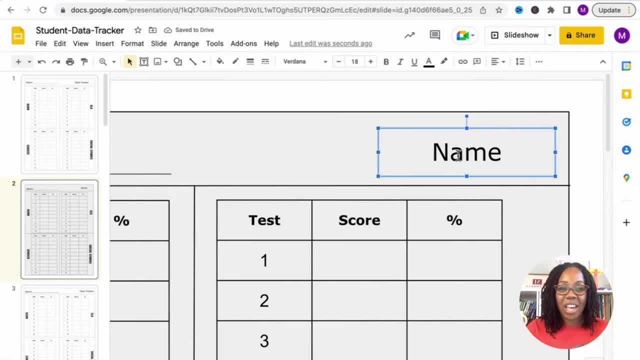 it's working enough. hopefully, you're getting the point. you're able to do this. getting the point. you're able to do this, getting the point. you're able to do this on your own, okay. so where it says name, on your own, okay. so where it says name, 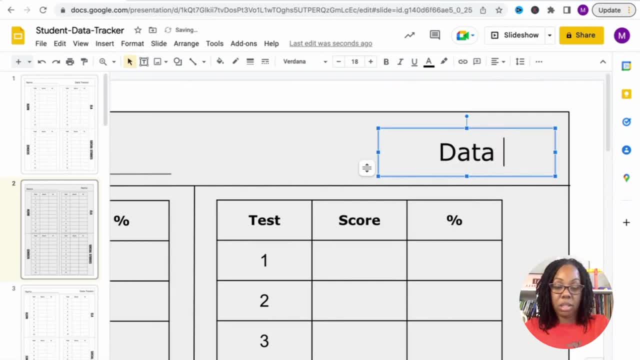 on your own, okay, so where it says name, we're gonna just switch that to data. we're gonna just switch that to data. we're gonna just switch that to data tracker. so we know what this is. or you tracker, so we know what this is, or you. 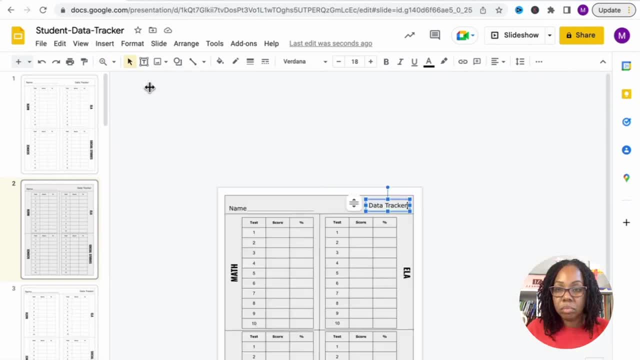 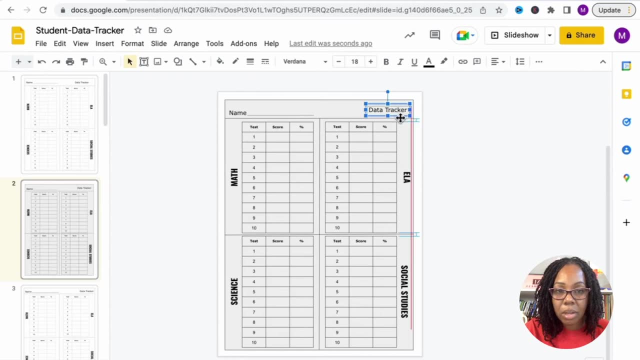 tracker, so we know what this is. or you know this space blank. I just like know this space blank. I just like know this space blank. I just like headings all right, and then we're gonna headings all right, and then we're gonna headings all right, and then we're gonna bring it down. okay, there it is, there's.